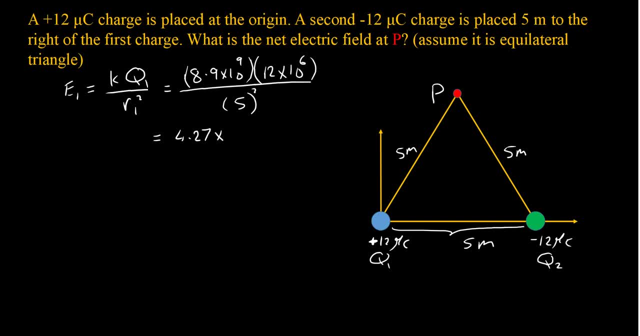 4.27, 10 to the power, 3 newton per column. now to decide the direction of the electric field generated by the first charge. well, our tested charge. we said it is a positive charge. we said that in our previous videos and this is another positive charge from q1. 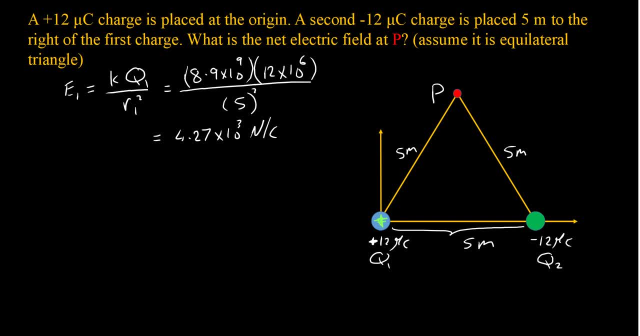 and that will you make. the electric field 1 goes this way, that's e1. now for electric field 2, which is the one generated by the second charge, it will be the same value of the electric field 1 as a magnitude, because it's the same distance. 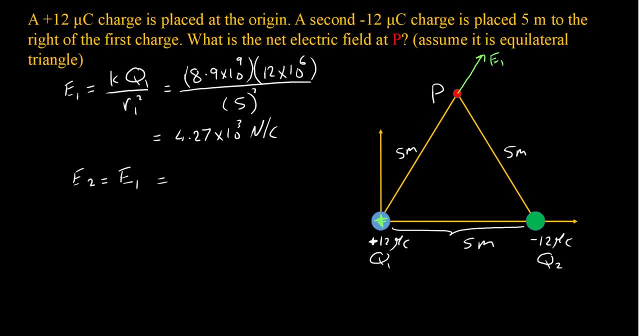 the same magnitude of charge, which means it will be 4.27, 10 to the power, 3 newton per column. but the direction of the electric field 1, 2 will not be the same as it is a negative charge, q2, that will make the e2 going downward this way. okay, so we managed to calculate the magnitude. 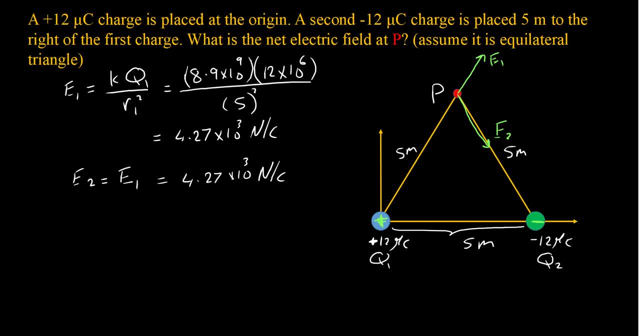 of electric field. 1, the magnitude of electric field. 2, the decided direction of electric field. 1 and 2. now to find the net electric field at point p, we should analyze our electric field vectors, try to change the color. so for e1 i will have e1 x. 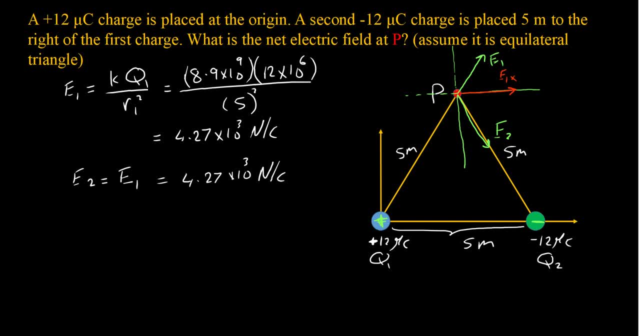 and also here it will be e1 y. let's pick another color. maybe we take blue for the electric field 2, that will make it e2 x and then e2 y. okay, now we can write them down quickly. so this is our exact e1 x. it will be. 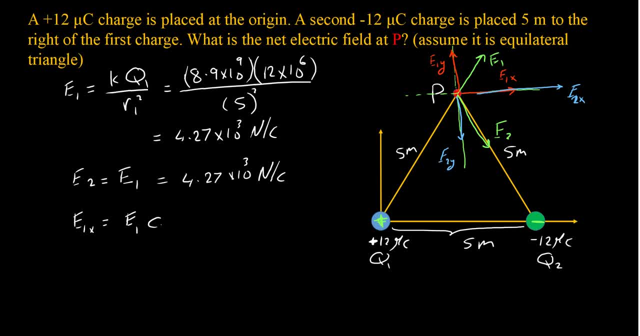 other e1 y will be e1 sine, 60 degrees for equal to a desktop illustrator. now you have to build our circuit. so what we have to right there is the Gy principe and heat node. so I am going to want y, which is going to be the endpoint for chocolate and blackjack and will look multiple wells and otherpan star him, etc. 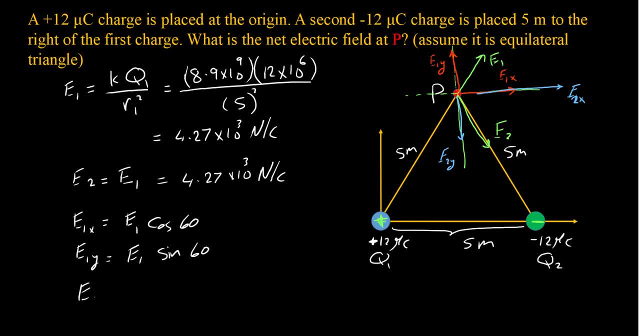 E2x, it will be E2 cosine 60 degrees. For E2y it will be E2 sine, 60 degrees. But whatever the value or the magnitude of E2y, it will come as a negative because it's going downward. 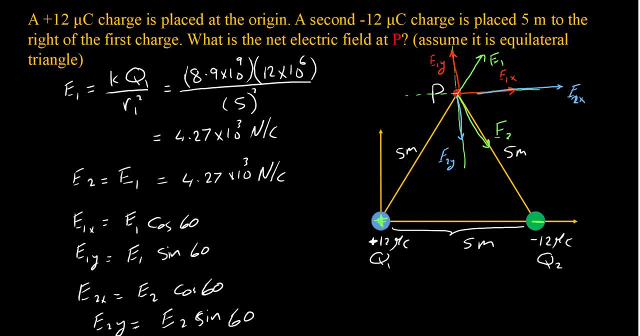 or it's going to the south or the negative yx. So, but you can see, because the magnitude of electric field 1 and the electric field 2 is the same and we're using the same angle, you can terminate for sure, the electric field 1. 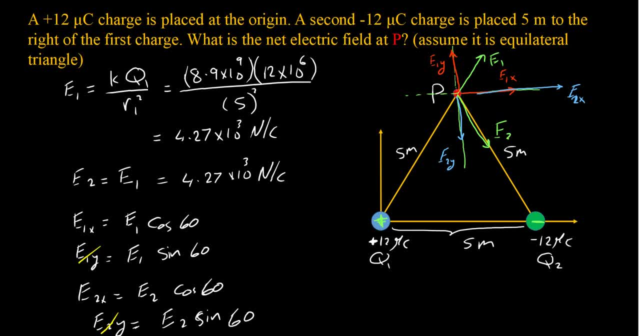 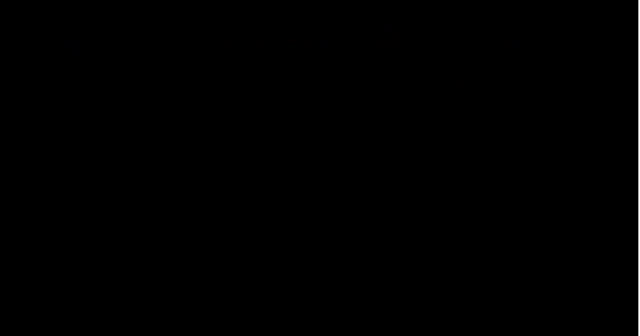 and the y component with the electric field of the 2y component, because they will be equal in magnitude, opposite in direction, which leave us with- I will end with that's our charge- P and I will have electric field 1x component. 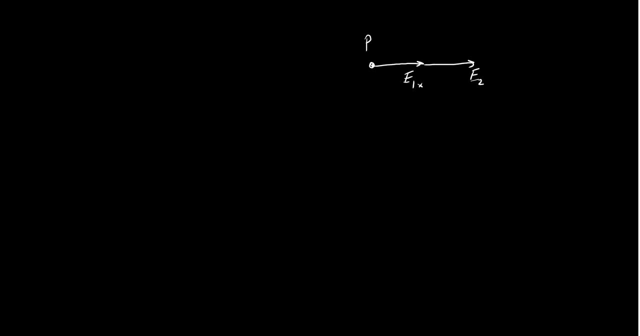 and the electric field 2x component, which means the electric field net it's going to be. it's going to be only on the x-axis, It will be E1x, that's, let's say, the total net electric field on the x-axis. 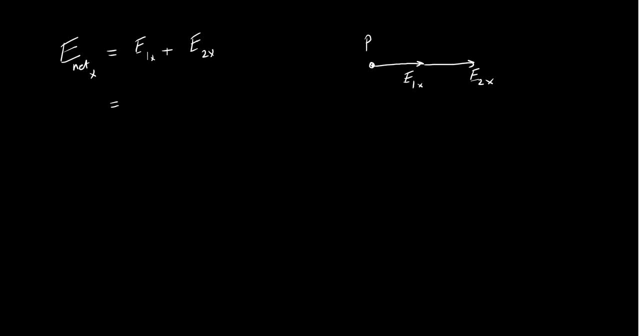 2x. that will give me, just to be more details, cosine 60 plus E2, cosine 60. They are exactly the same amount, So it's kind of like you times 2.. That will give me back 4.2710 to the power, 3 newton per column.